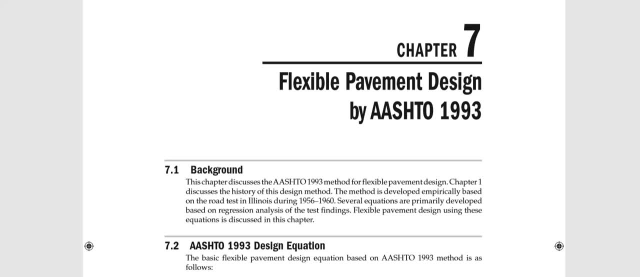 But still, though, we need to learn this method. There are several reasons behind that. The first reason can be: if you learn this method, then you will see the improvement when you learn the new method, But this is not an important reason. Other reason is that pavements that were built 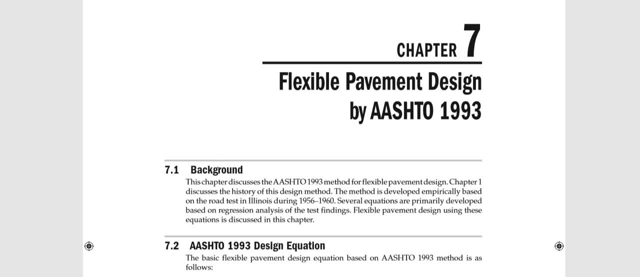 five, ten years ago, those pavements were built based on this method. So when you will work with those pavements or rebuild those pavements or redesign those pavements, you may need to know that method to see how the pavement was at that time. 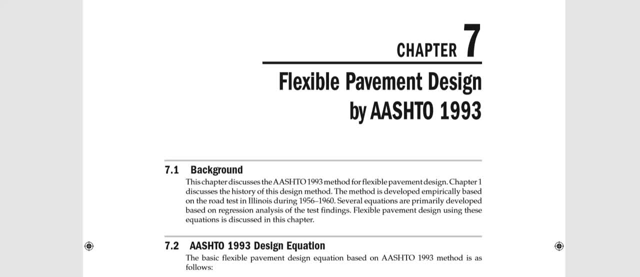 And then other reason may be still, though: some local pavements or some non-important pavements may be designed based on this method. So this method may be still useful if you would work in this industry. So let us see what this new method is. This method is: 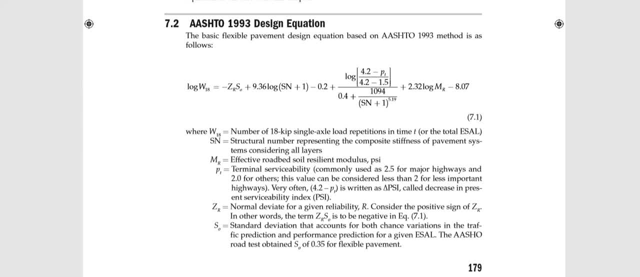 all about this equation. You can see this equation. So it's all about this equation. So in this equation, the left side is our demand: W18,. that means simply the total ESL, the total number of equivalent single axle load, Maybe two million, ten million, fifteen million, whatever it is. 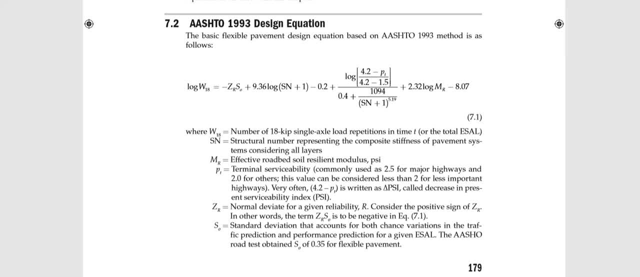 And right side is our capacity, capacity of the pavement. This equation looks very complicated but very simple. I am explaining one by one This portion. this portion is reliability. Es0 is the standard deviation of the performance that was observed in the Yaschow road test in Illinois. 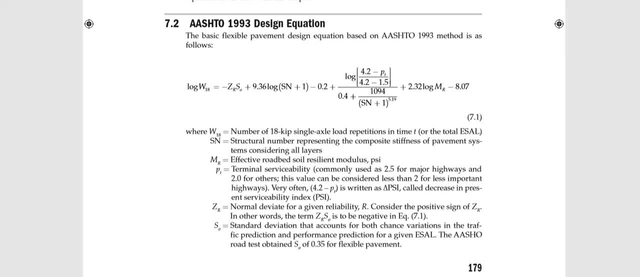 And zr is the standard normal divide, Normal divide. it is nothing to understand is simply read a value from the table based on the reliability. say, if you are design the pavement for 90% reliability, you have to take the normal debate for 90% reliability. now I will explain it again. 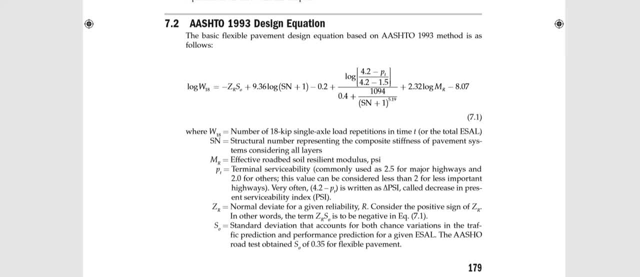 every time more details. so if you have confusion it will be clear after sometimes. then this is log SN. SN is the structural number. that is the output from this equation. in this equation everything is input, only output is SN. you need to calculate SN and then here P T. P T means terminal serviceability. what 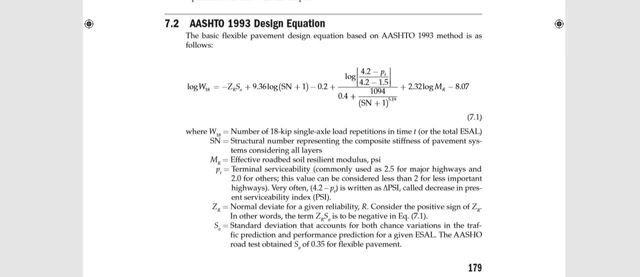 is this. it means the condition of the pavement and based on the scale from 0 to 5, 0 means actually the pavement is totally destroyed and 5 means so far is smooth pavement. you can see here we used 4.2. that means when we build a new pavement we are telling that the serviceability 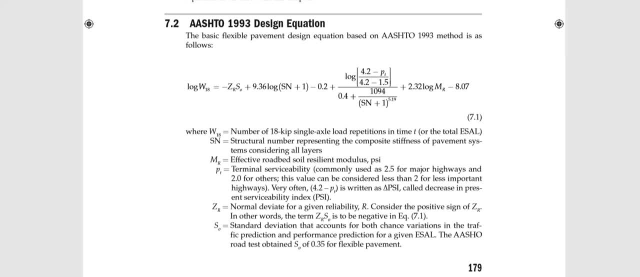 of the pavement is 4.2 out of 5. the reason, the reason that we did not use 5 is that we cannot build super smooth pavement, or super smooth pavement is not good for riding a car. we need some resistance in such. we need some friction to avoid the skid resistance. so when we 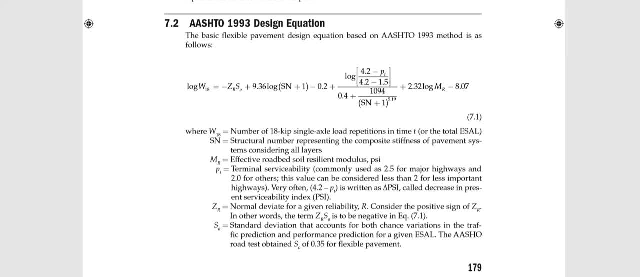 build a pavement that is 4.2. now what is 1.5? 1.5 means very low number. the pavement is failed, like pavement fail. you cannot be used anymore. so in that scale, what is your terminal serviceability? so you can say my terminal. 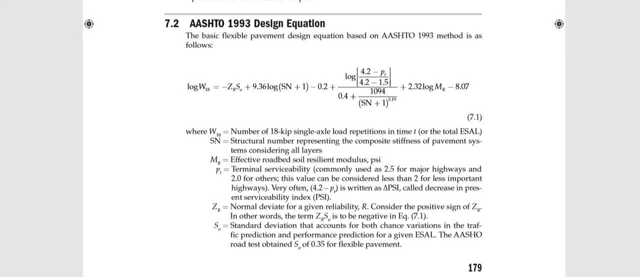 serviceability is 1.5. 1.5 means a pavement is totally destroyed. not totally destroyed means 0. so 1.5 means the pavement is there but it is impossible to drive on it. to give you some idea for inter-ester pavement, typically 2.5 is a good number for highway type pavement. 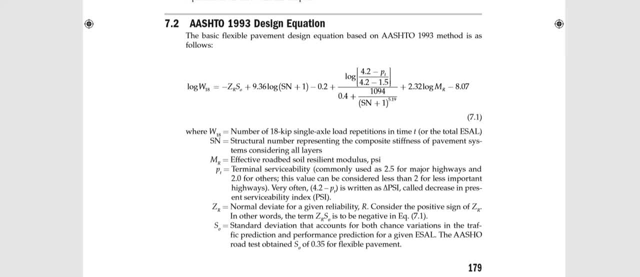 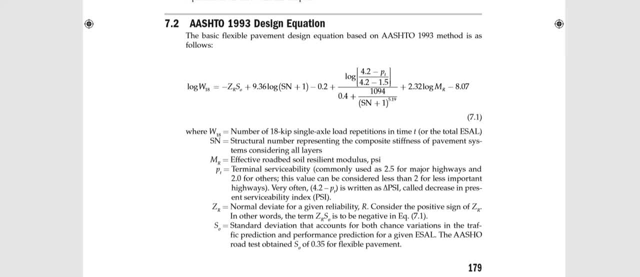 the resilient modulus of the soil or underneath the layer. so we will insert them. resilient modulus of soil, our desired terminal serviceability, that means at what value we want our pavement to be called failed. and then some reliability. reliability factor- and this is standard deviation is standard deviation is pretty known- is 0.35. yes, I wrote somewhere here. 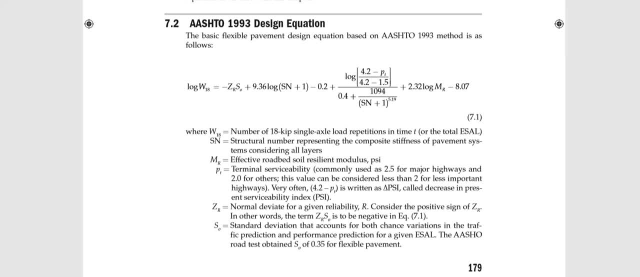 and this is 0.35. yes, I wrote somewhere here and this is 0.35. yes, I wrote somewhere here, and this is that totally sell the traffic level. so use this equation, find SN. that is the design output from SN we can calculate the thickness of different layers. how I will. 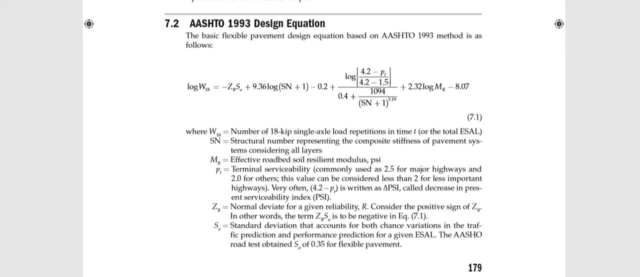 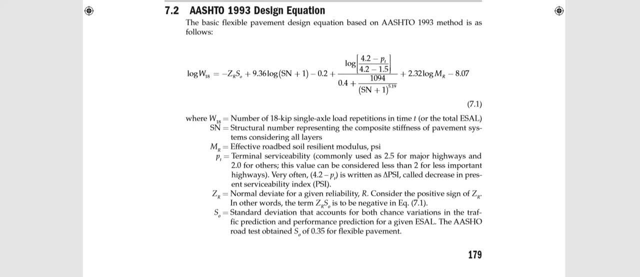 show you later of this chapter. okay, now we, we will do. you can see that this equation is very complicated, but there is a shortcut. what is that shortcut? come here, next page. so this nomogram. this nomogram will help you to calculate the thickness of different layers. 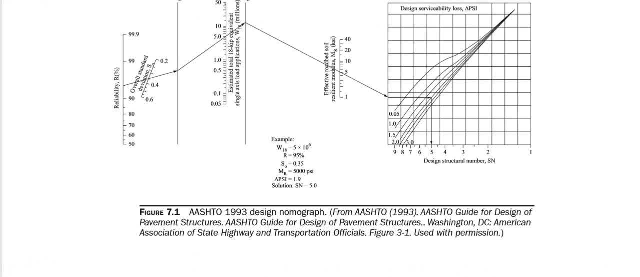 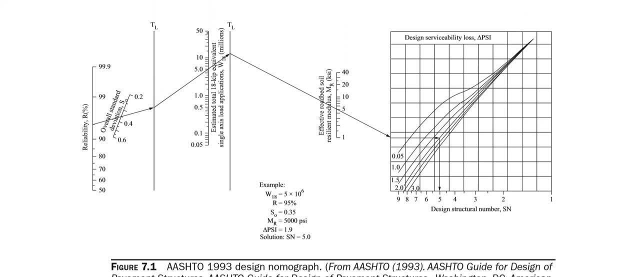 so this nomogram? this nomogram will help you to calculate the thickness of different layers. 0.4- 0.4. it will help us a lot. how is this option? 0.4- 0.4 hits 0.4. it will help us a lot. 0.4- 1- is this number cooked up? if I zoom in, you can see. so this nomogram will just solve that equation. that equation is very complicated to solve using this calculator, but if we use these one, again, very simple. how okay, start from here. reliability: what is your reliability of the by-bye patient? mostly we design payment based on ninety being designedtime. 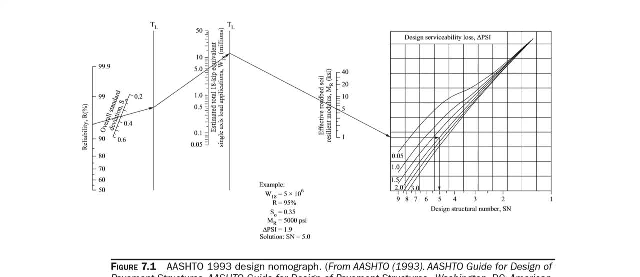 here it is 98%, whatever your reliability is, and I know that hopefully you know what is reliability. that is a statistics term. I'm not explaining or I'm not taking time to discuss that, but, very briefly, reliability means what is the reliability of your data like if we use a 90 percent reliability? 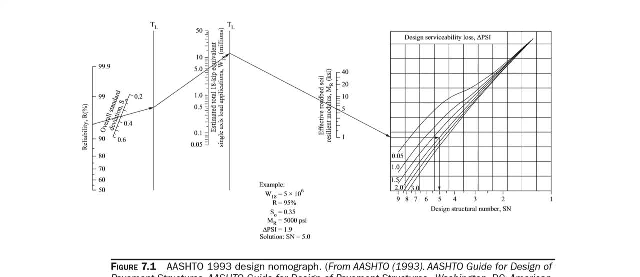 that means 90 percent of your data may be true. the 10 percent may be wrong. okay, so here it is 90, whatever, 90 or 98, whatever. then first use this value, whatever is given, or whatever your is your target. then external deviation is commonly 0.35, only 0.35. so if it, 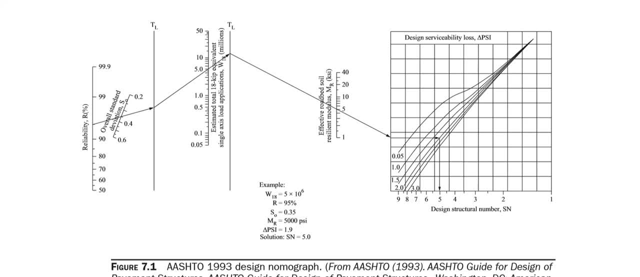 is 98 and connect this line up to this, then okay, then come here. what is your estimate, a total ishell. so if your ishell is, say, 50 million, then it is here, 10 million here, 5 million here, 1 million here. so locate your number. once you locate it, then connect your this point and 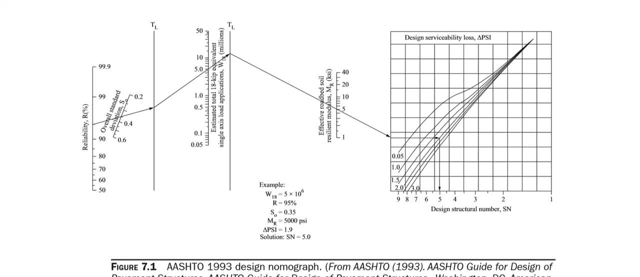 that point and go to up to this. then come here: what is your resilient modulus of the soil? so look at that point and then connect this and that. then go straight to here, then here to horizontally, come to this point. this is your delta psi. delta psi means a 4.2 minus. 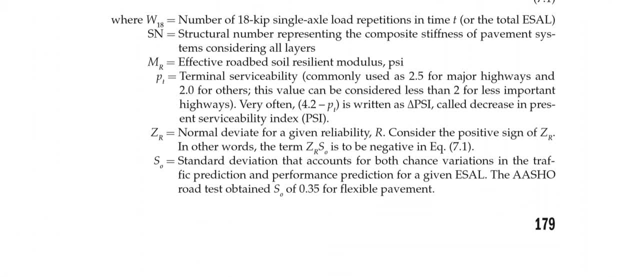 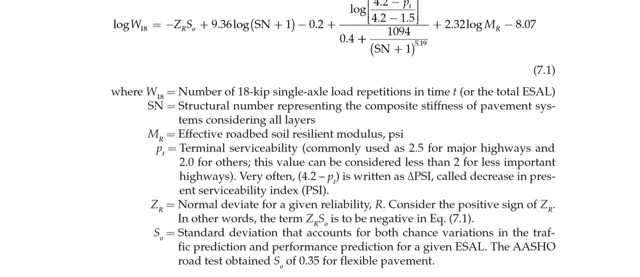 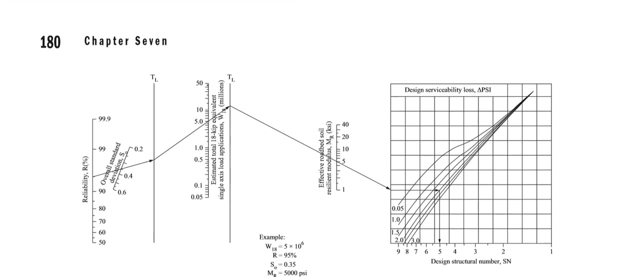 your solvability. that means the upper portion, the upper portion of this road, 4.2 minus minus pt, or that is also called delta psi. okay, you can see here, delta psi is 4.2 minus pt. okay, so go to that equation. sorry, go to that chart now. once you locate that point, then go down whatever the value is. that is. 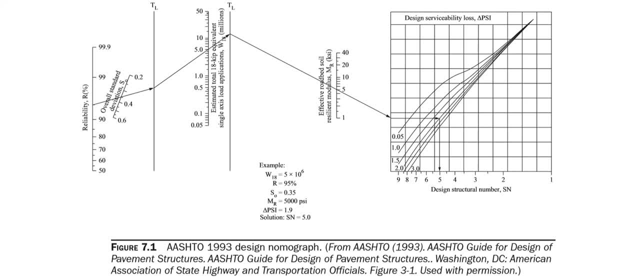 the structural number. so hopefully you you learn how to use this nomogram or how to use that equation. i do not recommend you to to use the equation because it is very complicated. you can use this nomogram now. once you find the sn, you can design your pavement. what to what to what to? 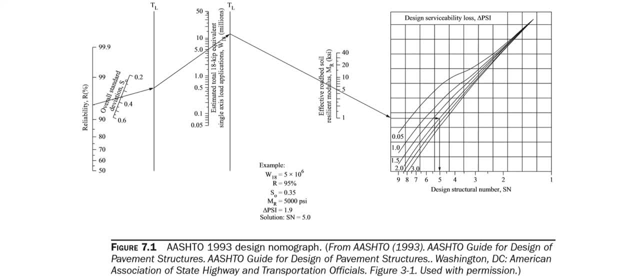 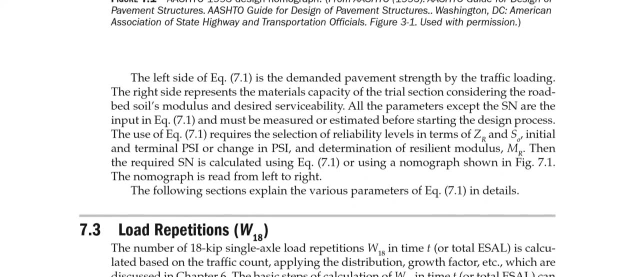 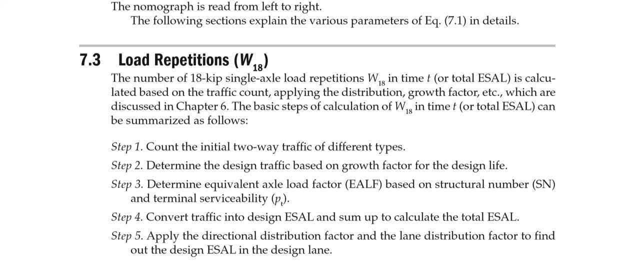 will be the thickness of the different layers. you can find it okay, we will see that at the last of this chapter. so now we will go one by one. first is w18. what is w18? simply, it is the total excel. whatever you learn in chapter 6, that is, first, calculate two-way. 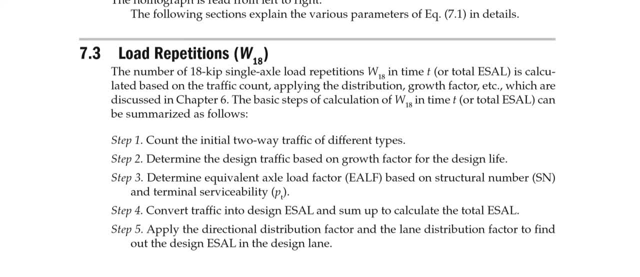 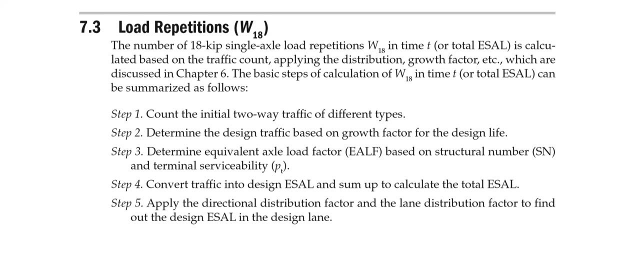 initial traffic, then forecast it based on the growth factor, then calculate the equivalent single equivalent axle load factor, then convert into esl, then distribute it, for you do not need to distribute it, uh, if you're um, no, no, you, you need to actually distribute it based on your. 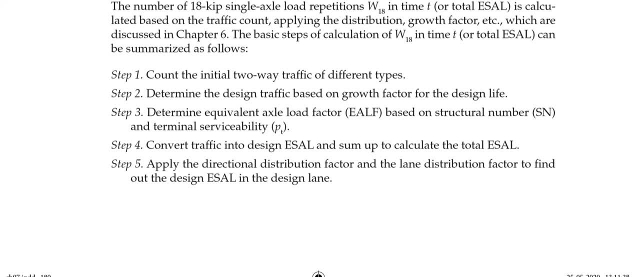 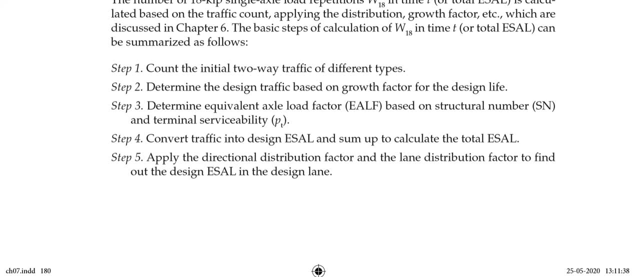 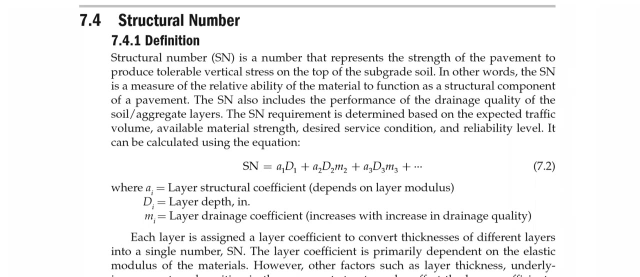 design length. so you can. you learn that also. you need to apply distribution factor and land length factor. whatever you learn in chapter 6 to calculate diesel is same thing. so w18 is nothing, okay. next is the structural number. what is that? structural number is just a number, but this number will tell the capacity of the entire pavement. 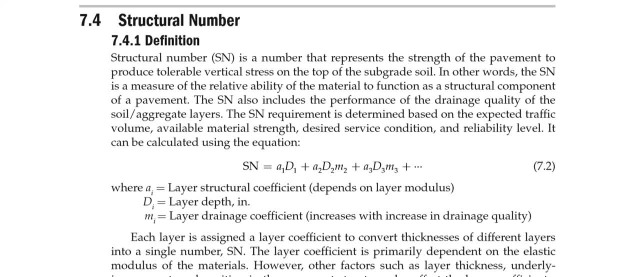 so, or simply the capacity of the entire pavement is called structural number. now how do we calculate it? see, sn is a1, d1, a2, d2 m2 plus a2, a3, d3 m3. what is that? a1 means layer coefficient of top layer. that number only. 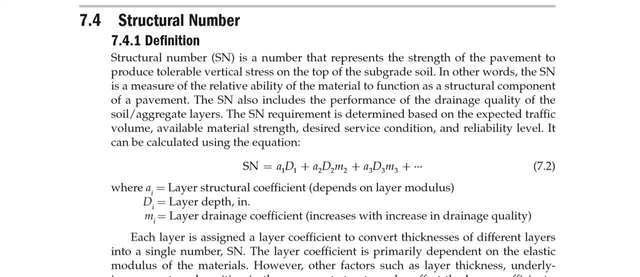 d1 means depth of that layer, so this one is um. d1 means as per layer depth, a1 means the coefficient. now, what is coefficient? the coefficient is a value from 0 to 1 in the scale of 0 to 1. what is the? 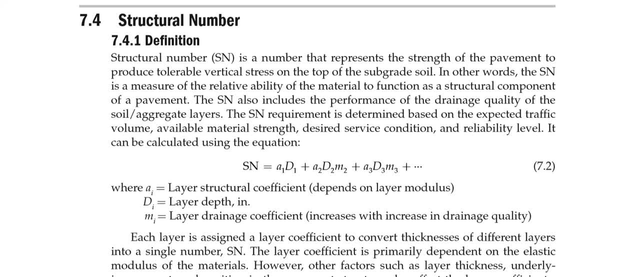 modulus inside this scale. so zero means simply water, uh, water or water type, and one means is full, rigid, maybe mild steel, but we are talking about flexible pavement. there is no mild steel still or is still here. it's in that scale, in that scale where your asphalt is- typically asphalt is. 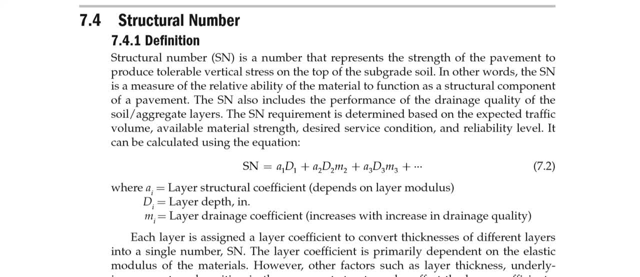 0.4, 0.44. like this and similarly here. base layer: a2 means a layer coefficient of base layer and d2 means depth of the base layer. m2 means the drainage capacity of base layer. if drainage capacity is good, we can consider this one then. similarly, this is for sub base. okay, so hopefully. 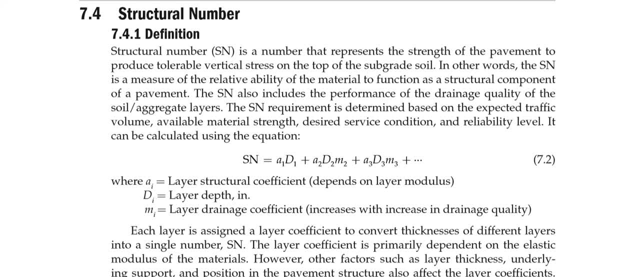 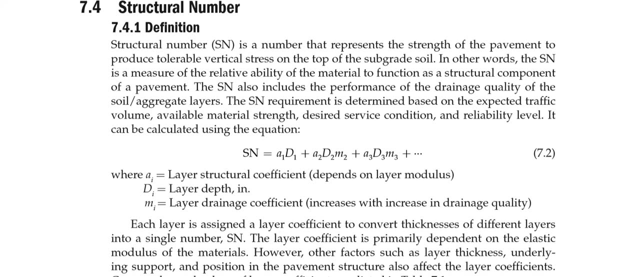 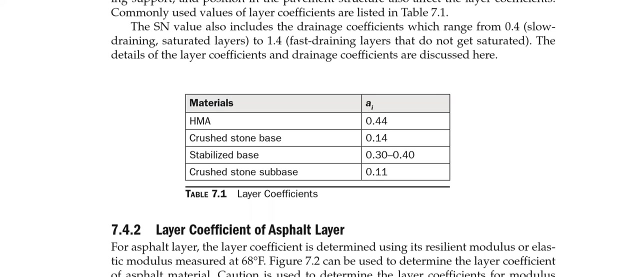 you, you learned it. now. this calc: whatever sn we we get from the nomograph, then we make it equal and then, based on different combination of this, we select d1, d2, d3. we'll know better in the last of the chapter. okay, now we will see how to. before going there later, some general values of the layer. 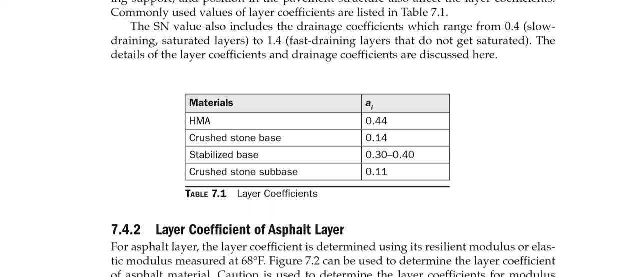 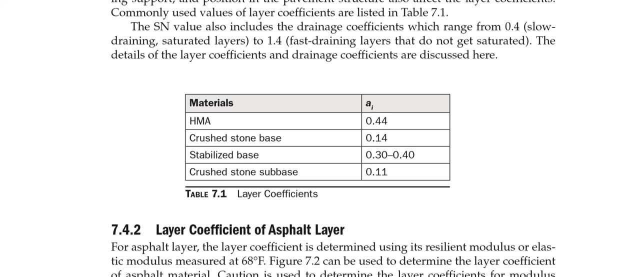 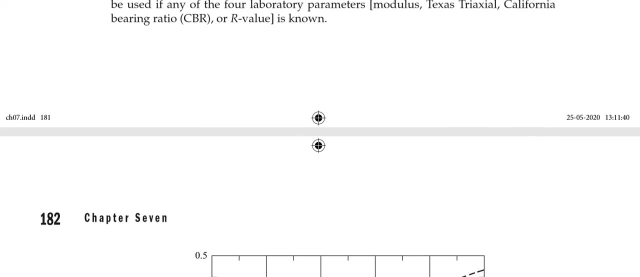 it will be 0.3, 2.4 and subbase is 0.1 on. so this is a typical values. now how to find a layer coefficient for asphalt layer. so, as per layer, we can find the layer coefficient using our modulus: the modulus. 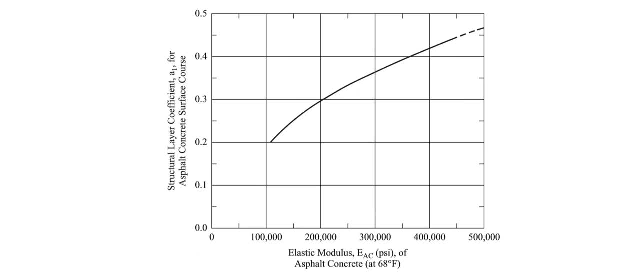 the elastic modulus of the asphalt At 68 degree Celsius. So at this temperature we need to determine the modulus of the asphalt concrete. then come to this table. Say: if it is 200 Thousand, then come here, go up and go left is point roughly 0.3. 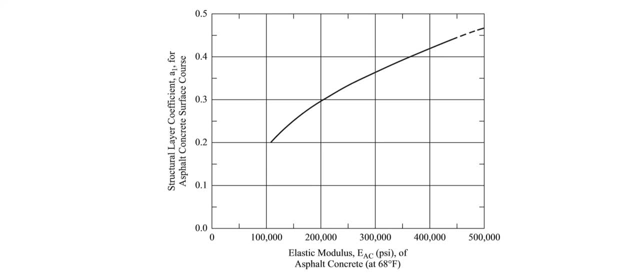 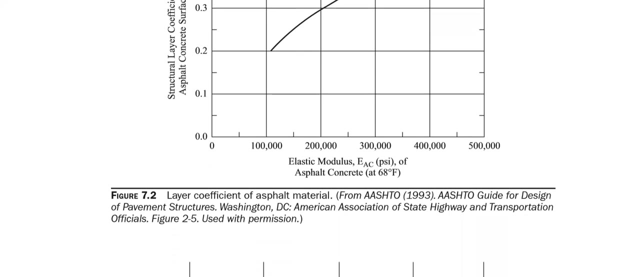 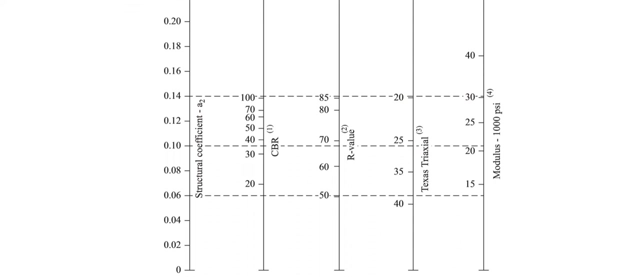 If your modulus is 400,000 psi, then come here, go top, then go left, 0.4243, whatever. So in this way we can find the layer coefficient for asphalt layer. Now how to find layer coefficient for base layer. So layer coefficient for base layer we can find many different ways. one is either find the modulus or find the. 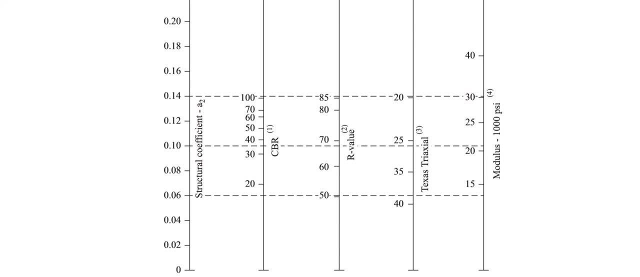 Texas drag gel test. find the number or find the R value or find the California band ratio, whatever you do. So whatever you do, then Say you you would did R value and you can. R value is 60, then come here. R value is 60, go left. 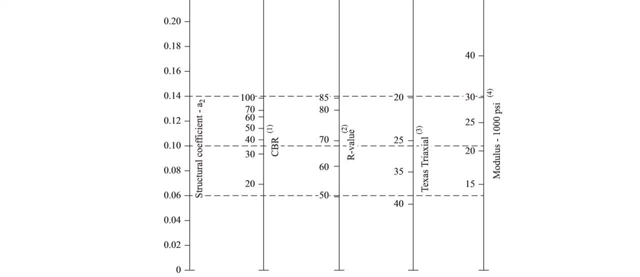 go left roughly 0.085 something. Say, if you are California, if you did California band ratio and it is 80, then come here, go to 80 roughly here, then coefficient is roughly 0.13 something. So whatever test you do, you can find it. 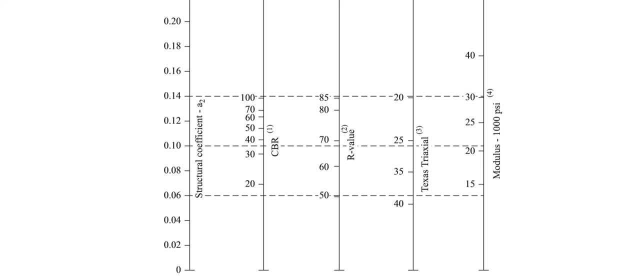 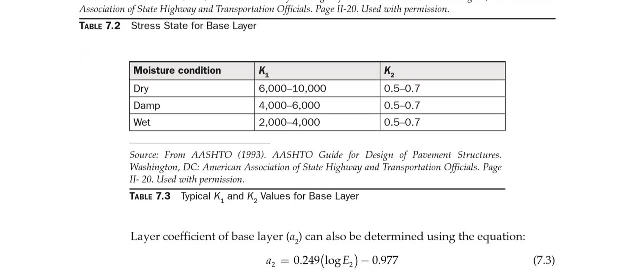 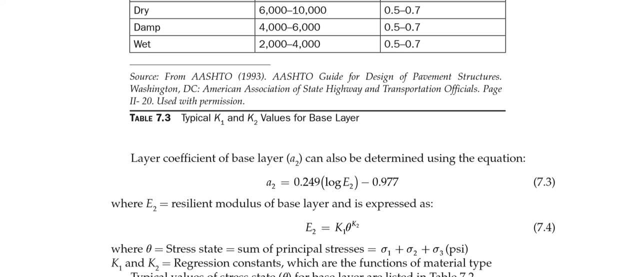 There's also other way to find the layer coefficient of base layer. How You can see here, there is some equation, Okay, some equation is this equation: So a2, a2 is 0.249 log e2 minus this. How to find e2?? You need to find e2 is k1, third to the power, k2.. What is k1?? 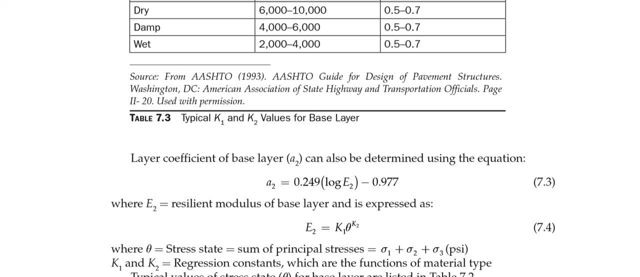 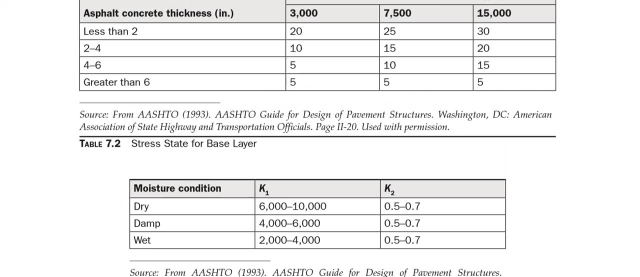 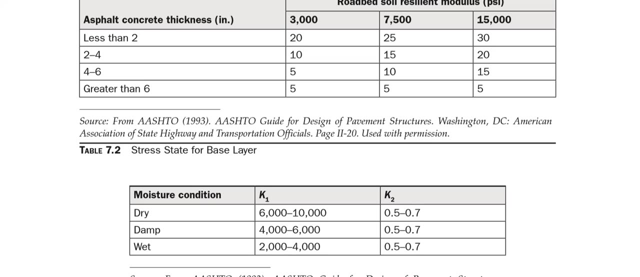 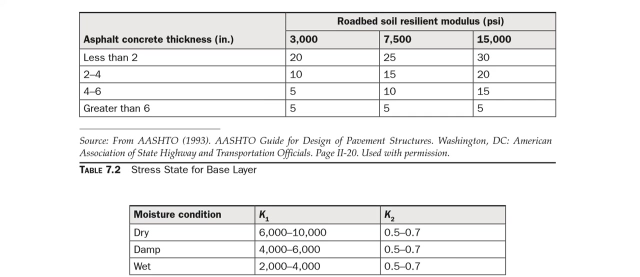 k1- k2. See, very simple. you do not need to do anything, just the table is given here, Table is given here, Table is given here. So, okay, Okay. so yes, you can see how to find k1- k2 based on your moisture condition if it is dry. 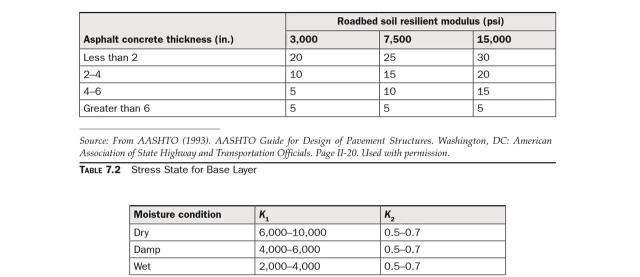 k1 ranges. between these you can take average number or whatever number. Then k2 ranges this: if your soil is wet, then this and k2. is this How to find theta? theta is based on asphalt thickness. say, if your asphalt thickness 4 to 6 is and? 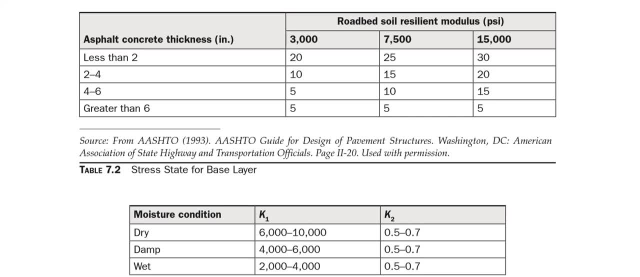 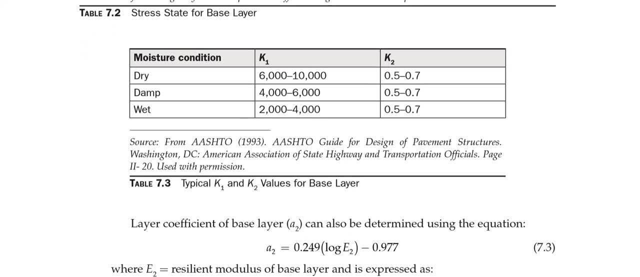 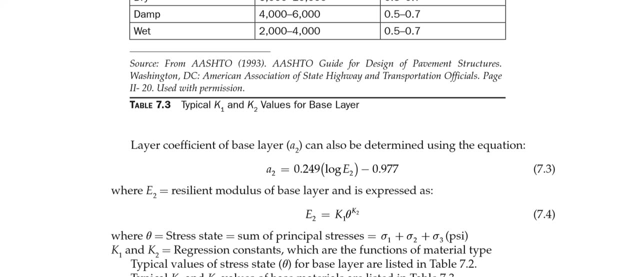 Soil modulus is say 7 and 1500, then your theta is 10. So you can read k1, k2 and theta from this table. insert it there. then you can find A2. so that is another way to find a2. So this is similar for sub base. for if I go down for sub you can see this example. 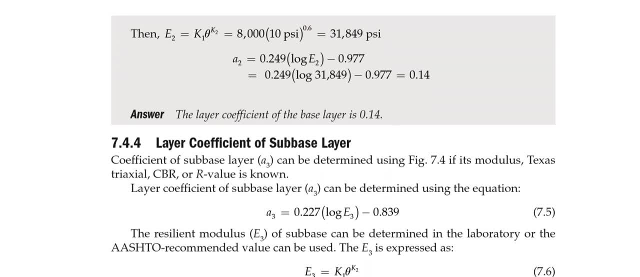 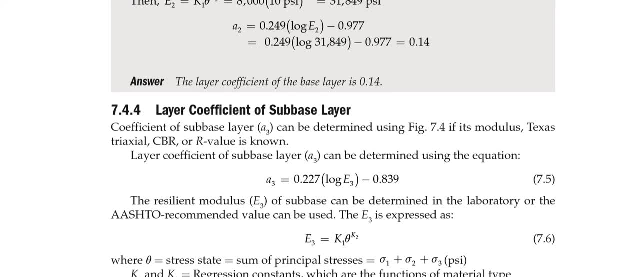 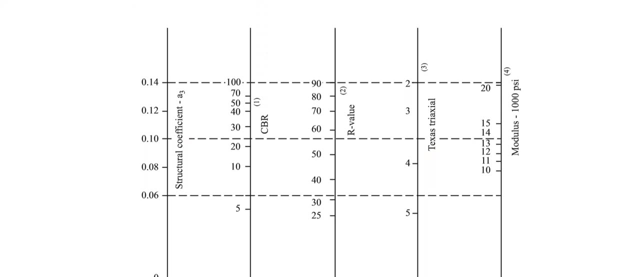 for practice For sub base: similar approach. you can use this equation. You can use this equation Or you can use the chart. This chart is based on your soil sub base, modulus or Texas Drexel test or R-value test or CBR test. then you can find a3 or you can use the above. 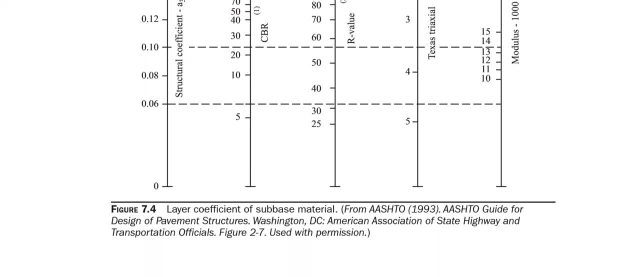 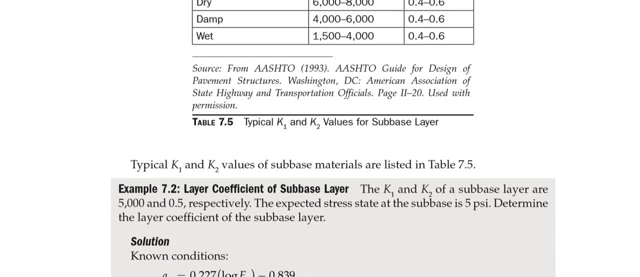 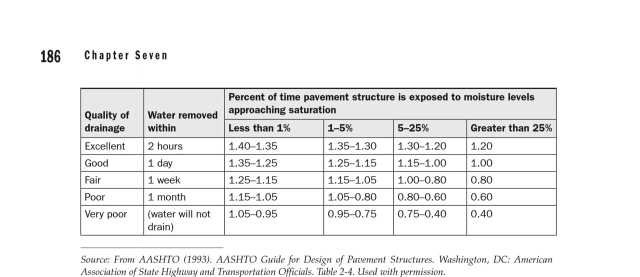 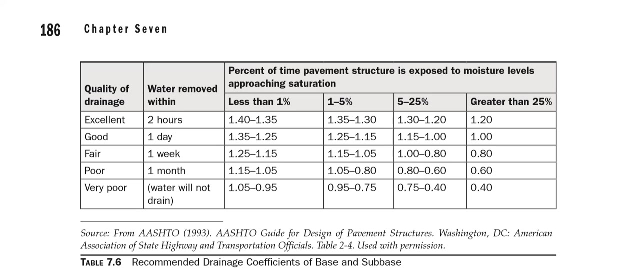 equation. So hopefully you learn how to find layer coefficient for different layers. And now we will go. There is another example: Drainage coefficient that means m2, m3, so drainage coefficient is based on this table. So based based on this table, say your sub base layer, The quality of drainage is, say good. What does good means good, means water. 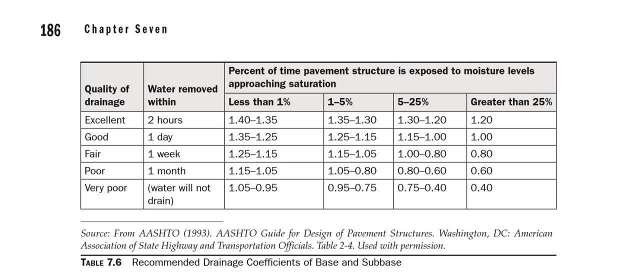 Water will remove within one day and we call it good Then. percent is of the time theTONY Structure is exposed to moisture level. That means they. if it is not in the rainy zone, the pavement may be exposed to rain maybe 10% of the time. bar 10% is very huge, you know. Oregon may be. 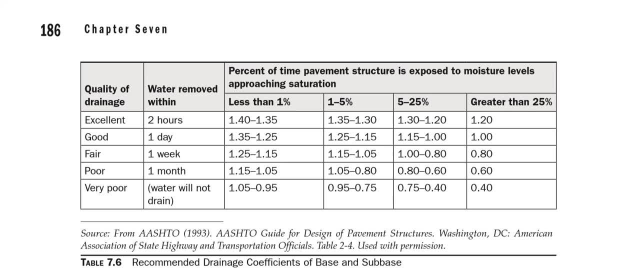 30%, 20% in dry area like New Mexico, Arizona, Maybe 1%, so that is the person's of the time your pavement will be exposed to water. So, based on on your quality and based on the time, you can choose your number: m2, m3. 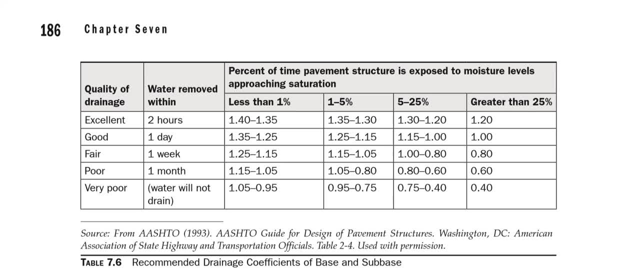 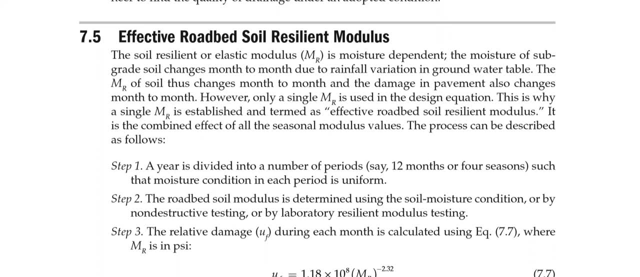 whatever. so this is the, this is how you can take and the number of, sorry, the value of m2 or m3- now, other value is M- or how to calculate AMR. so simply, you can take a sample, take it to the laboratory and determine the modulus it's. 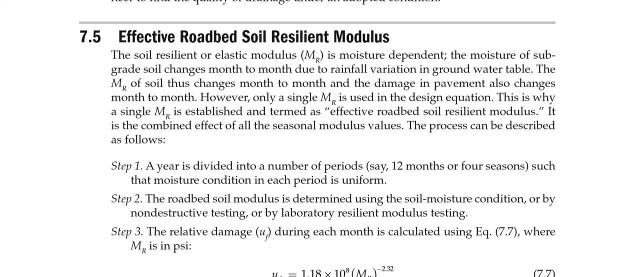 very simple. but it is not so simple because you know that the modulus of soil depends on the moisture condition. if moisture is high, modulus is less. then how to find a single value in that equation, the beginning, the equation I showed you big equation: it uses a single value but the modulus of style changes. 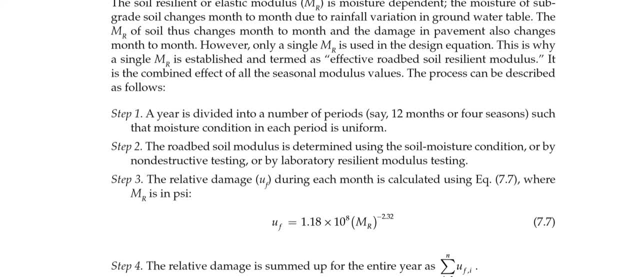 with seasons. so what, how to do? what to do? first, we divide the season. you different number, say 12 months, or you can say: for summer, winter or winter, 차 sorry. spring, summer, fall, winter. for season, you can divide it or you can divide by 12 months. 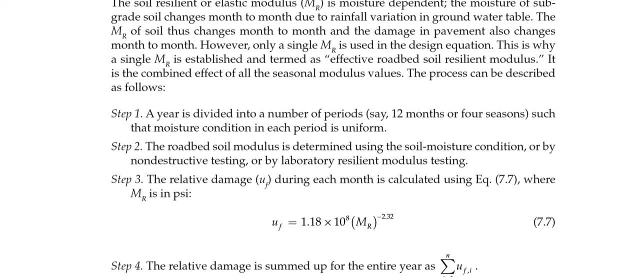 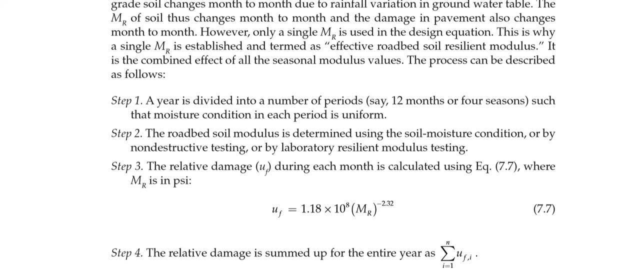 or you can divide into 52, 52 weeks, and based on that, for every times their moisture in the soil will change. based on that moisture calculate modulus. but if we do, 52 is huge. so 12 is a good number. every month one. so every month in that region. what is the moisture? moisture level based? 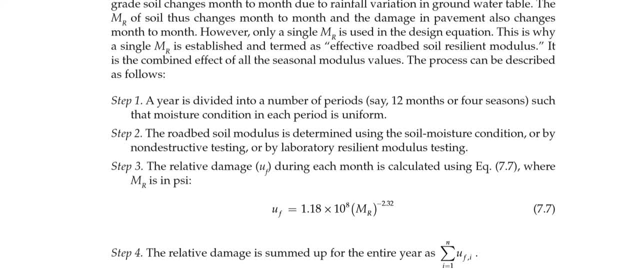 on that moisture level, find the modulus okay. so first we divide the year into different numbers: 12 months or four season or three season or two season or 52 weeks, whatever you like- then determine the soil modulus for that different season, then calculate a relative damage. relative damage means if your modulus is high, the damage in the pavement, for particular. 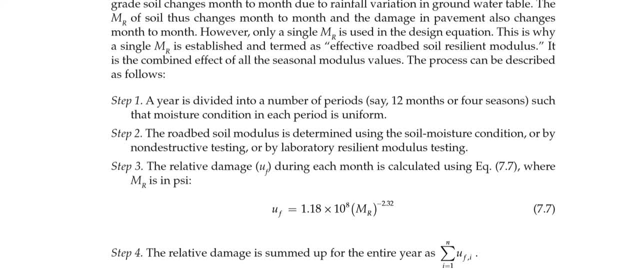 load will be low. so that is called relative damage. so it is a empirical, empirical number. so empirical number it's for empirical equation, empirical equation. so used using this calculation determine relative damage for different period or different months. whatever your division is, if you sum up you will get the damage for entire year. then divide by 12- no, actually not 12- divide by: 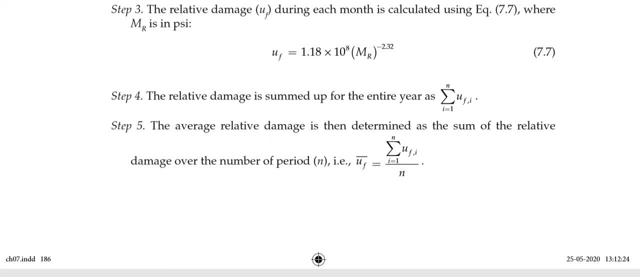 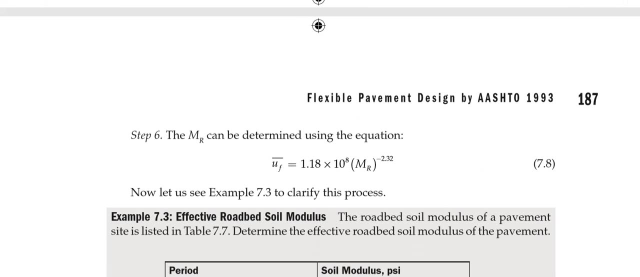 the number. if you divide by the number, you will get the average damage. you will get the average damage. once you get the average damage- average relative damage- then use that equation again to back calculate the MR. that is how we calculate the value of MR. okay, so there is an example here to understand better. I know that it looks very. it looks very. 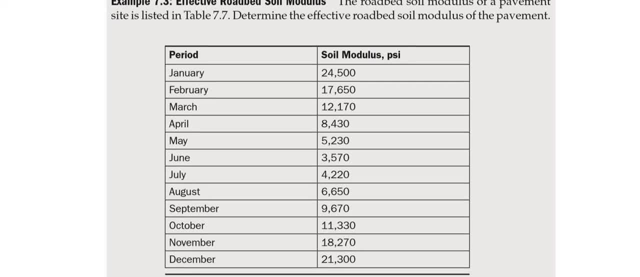 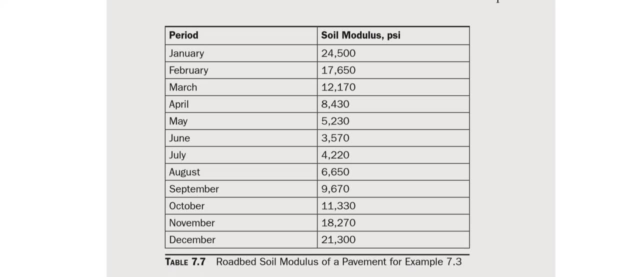 complicated but very simple. say here: we divided the year into 12 months. every month we determine the most. we collected some sample and determine that soil modulus. so these are our modulus, so the average modulus. then we will calculate what is the average modulus. so average modulus is not the 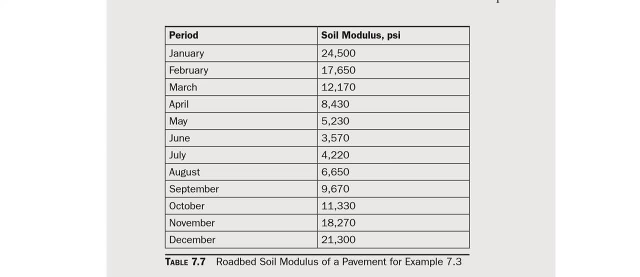 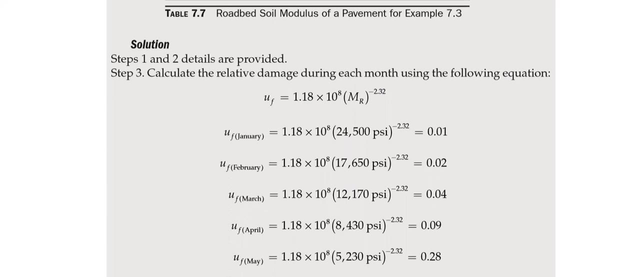 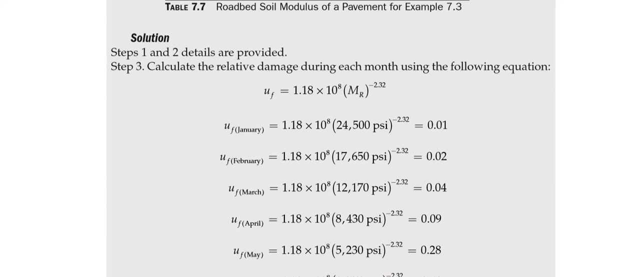 average of the such as this: it should be based on the average damage in that pavement. so what we'll do, for every month we will calculate. so for every month we will calculate the relative damage, say relative damage in January, these February, these March, these after calculation. I don't know why my cursor is not working. yes, now it is. 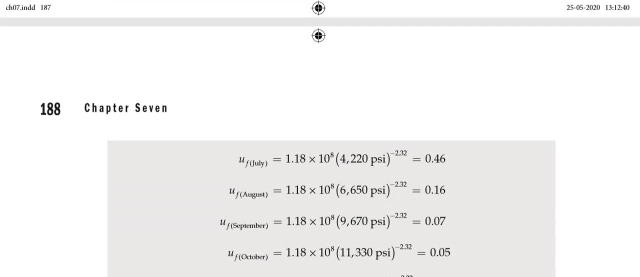 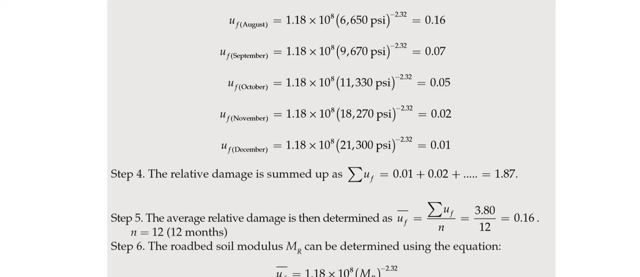 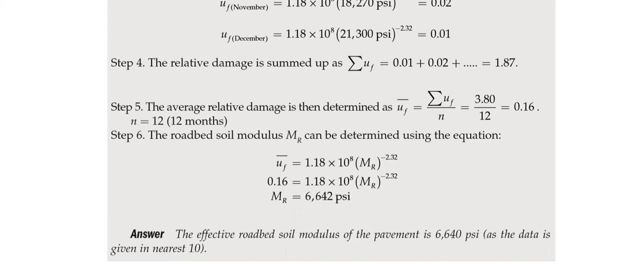 working case. you can see defined months. we calculated relative damage. after calculating we summed up all, then we divided by 12 and got the average value. once we got the average value, we use the average value here and calculated our modulus. so that is the effective roadbed soil modulus. it is the average. 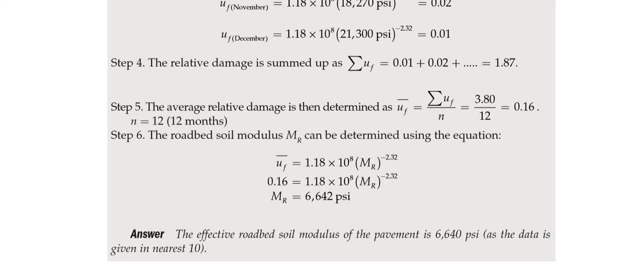 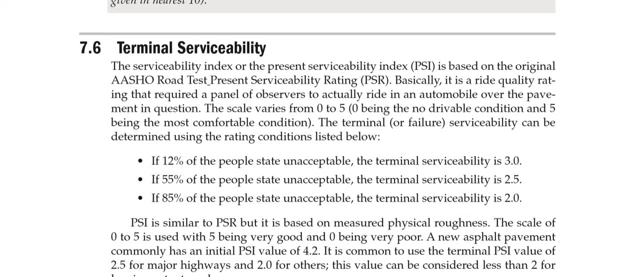 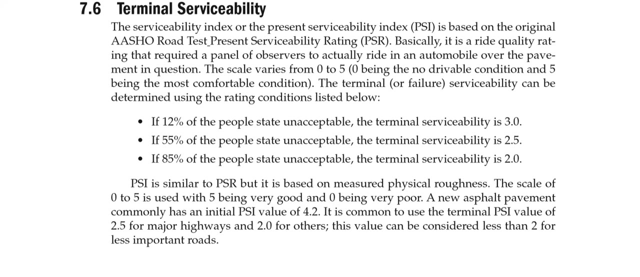 of all 12 months, based on the damage. so this is how to find effective roadbed soil modulus. other term is terminal serviceability. so yeah, I already discussed it. based on the scale of 0 to 5, we give a number and that if my pavement decreases to this, we will assume it is fail. 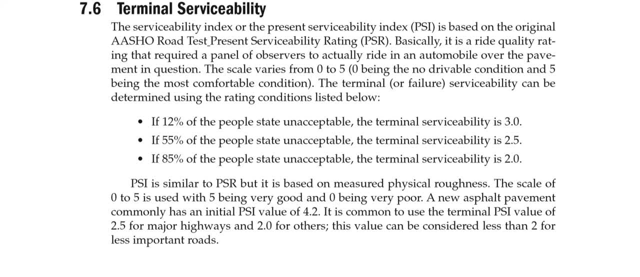 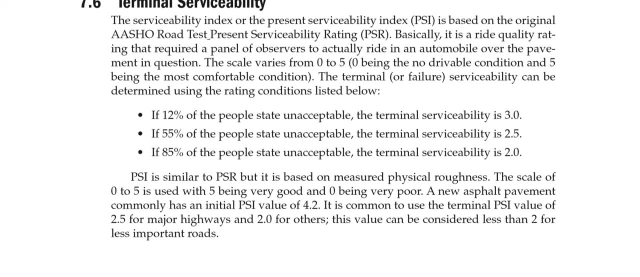 you okay. so how that number was developed, that if it is 1.5 it is failed based on this assumption that if 85% people say the road is unacceptable, that means that condition is true. if 55% people says the road is unacceptable, that means that is. 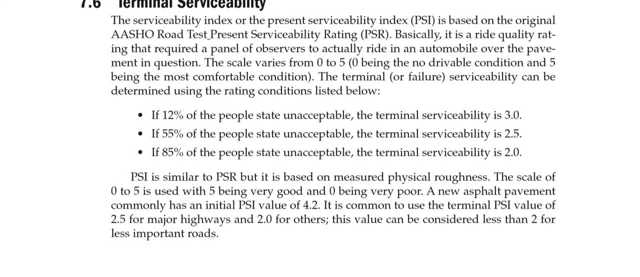 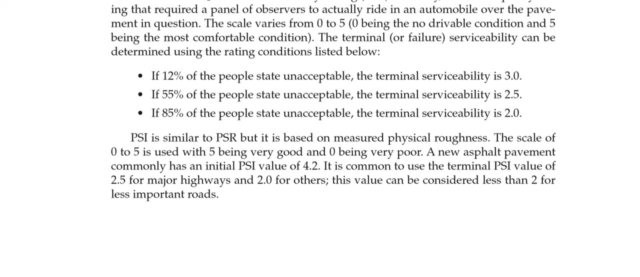 2.5. so based on this, like logic, it's not exactly, nobody can tell exactly: pavement fail, somebody will fail. so that is the assumption that if the road is unacceptable, somebody will say fail, somebody will say no. so based on this assumption, and I told you it is a common, like common or general value for interstate 2.5 is a. 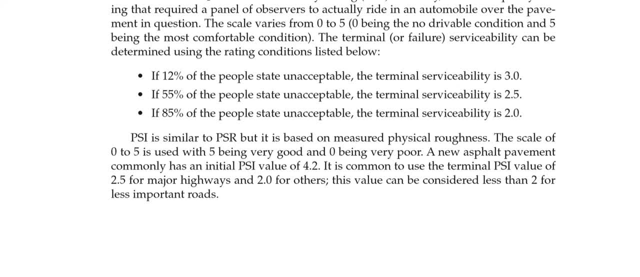 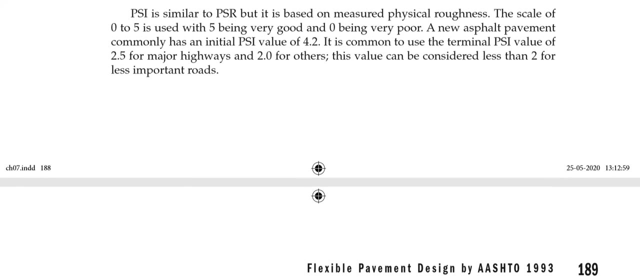 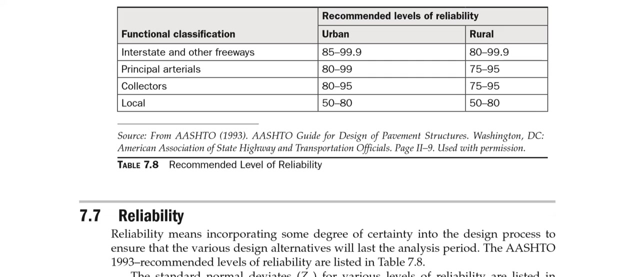 good number to assume: terminal serviceability for major local road to for normal, non important or very residential road may be 1.8, but again, it is based on the demand of the public. now, reliability for reliability. what should be our reliability as to give us some guidelines. if it is interstate and urban area use 85% to 99.9. if it is, 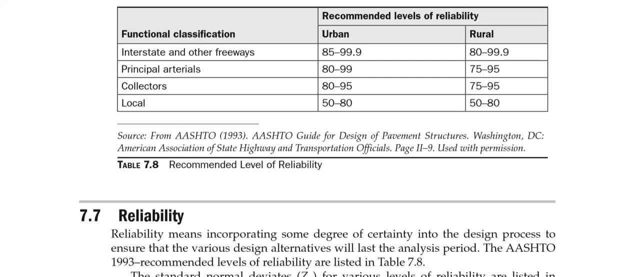 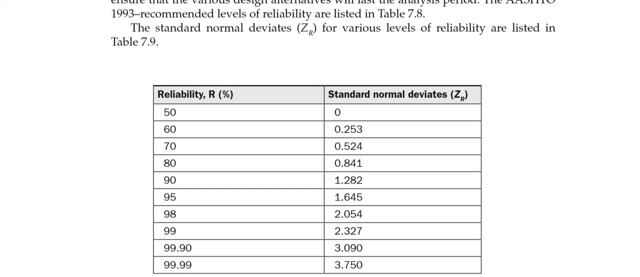 local, say for urban area 50 to 80, rural area 50 to 80. also, that is some guidelines. you may not follow this, no problem. then what? how to calculate the divide? at the beginning i told you: uh, you need to know this. what is? that is simply table, if your 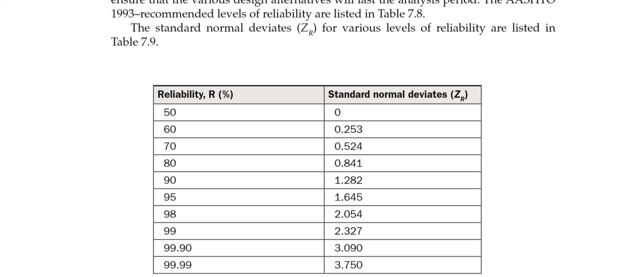 reliability is 90 percent, then your gr is 1.282. we design pavement mostly for 90 percent reliability, so better to memorize this value, or sometimes 90 and mostly 90 percent. if it is 98 percent, 2.054. so now you know what is normal divide is. it is based on the normal distribution. 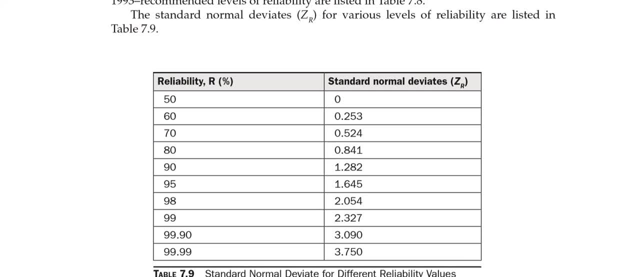 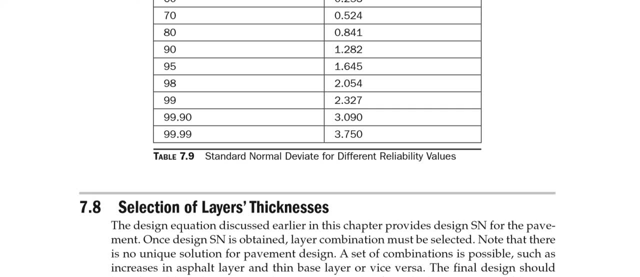 that you saw it in your statistics class. okay, so we discussed the initial design equation or design nomograph, and i discuss every term very briefly. you can read the book to learn more. yeah, i'm going very fast because if my video length is so big, nobody will watch it. 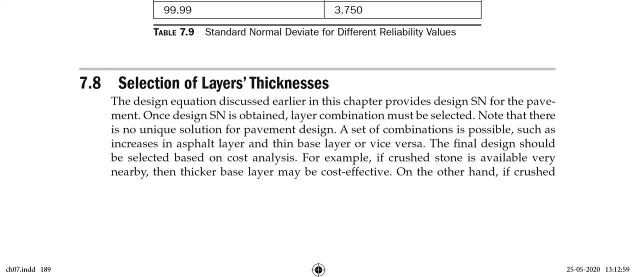 so i'm going slow. now, after learning all this, this is our final learning: selection of layer: layer thickness. how will we select our, or how will we design the pavement finally? so this section is very important. okay, in fact, we discuss it, but now we will apply our knowledge. 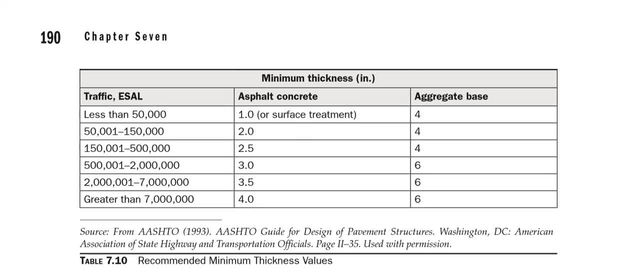 before starting, this table will show you what is the minimum thickness possible. so, after designing, if you see that your asphalt thickness is, uh say, for this case when your cell is two to seven million, you found that your asphalt thickness is twins. but you cannot be it. you cannot use less than 3.5 is. that is the astro recommendation based on this method. so 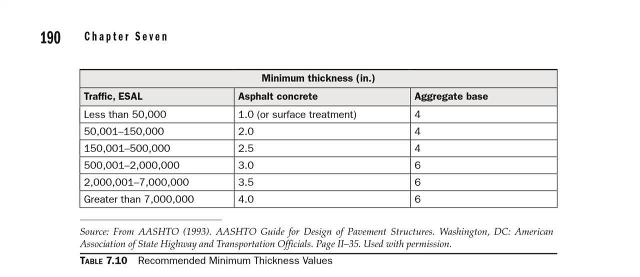 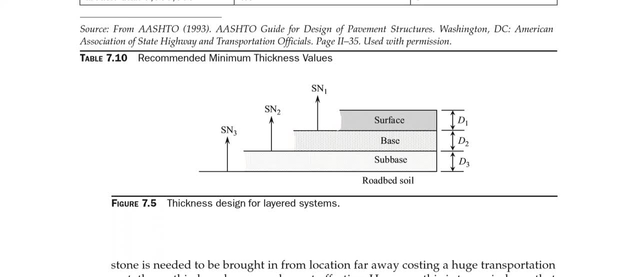 whenever, after your design, you should shake it with this table that it cannot be less than that. okay, so this, this figure, will explain the method. so what we will do at the beginning. at the beginning, we will assume that our pavement will have only one layer, only this layer, not this layer. we will neglect this at the beginning. we 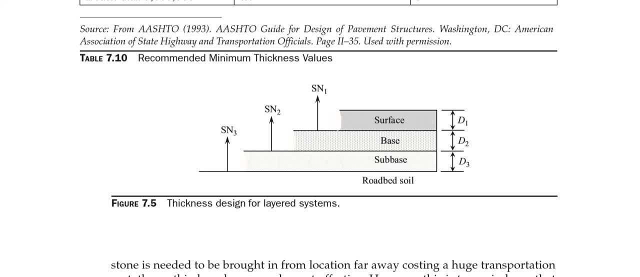 will assume our pavement will have only one layer, then we will, and the modulus of this will be our again. i am repeating because it is important. so at the beginning we are assuming that this is our soil, this is our soil and it is infinity. then this is our mr, and then we will calculate our. 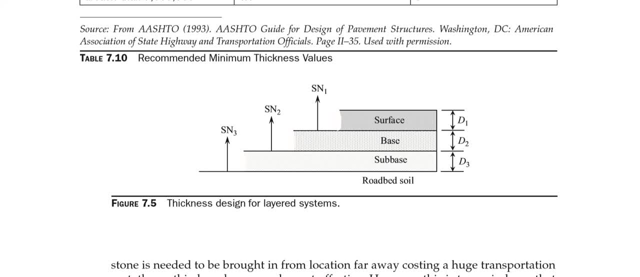 sn. how you will calculate sn? based on the initial equation, the first equation i showed big equation, or you can use the nomogram. then if we use, this is your mr, the mr, here is your MR, and if you find SN, then your SN1. one means like first layer, so your SN1. 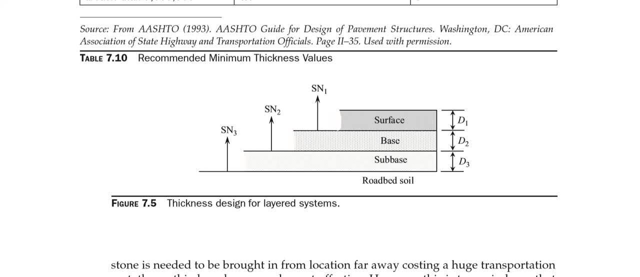 will be equals A1, D1. so if you know the A1 of this layer you can find D1. so that is the way to find D1. then choose a round number. once you find D1, then assume the modulus of this is your MR. then calculate or find SN2, SN2 will 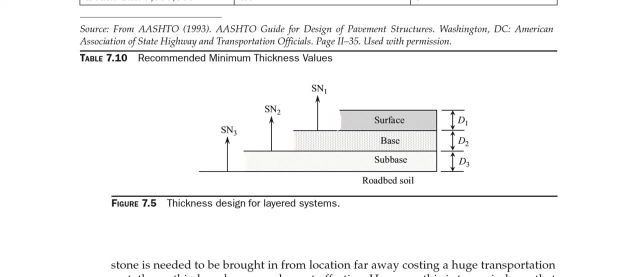 be A1, D1 plus A2, D2, M2. so you know A1, D1 for this. now you know A2, M2, then you can calculate D2 here. then take a round number, then come here. this is your MR and you can easily find and mark it here. 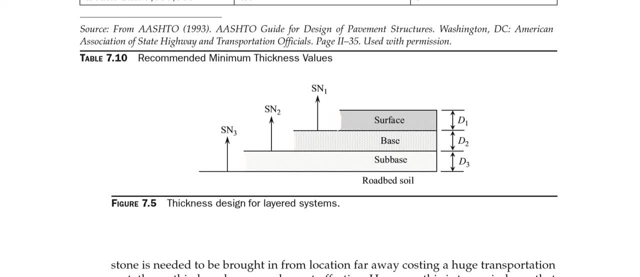 Calculate SN3. Then SN3 will be A1, D1, A2, M2, D2, A3, M3, D3. You know this one, you know this one, you know A3, M3 for this. Then you can calculate D3.. So this way you can calculate. 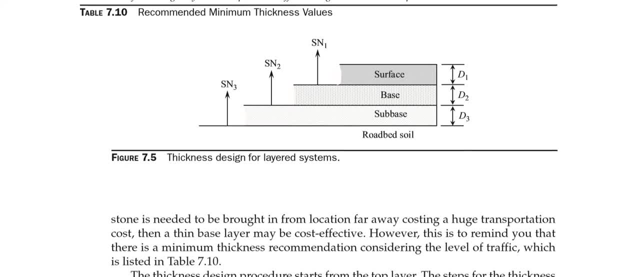 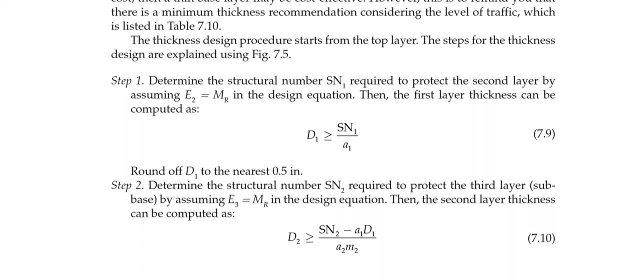 different layers thickness, one by one. So I explain this here by step by step. So step number one: assume your E2, that means the modulus of layer 2, as your MR, Then use the equation or the nomogram and calculate SN1. Then your D1 will be SN1 divided by A1. Then whatever you will get, 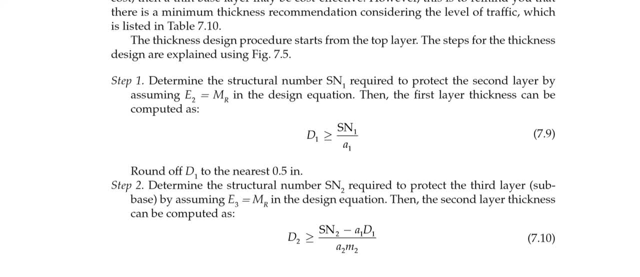 take a round number. This bigger means it cannot be less than the required. You can take a higher number. So you got 6.1 D1. Then use 6.5 or 7 inch to be a round number. So the yearbook said that round D1 to nearest 0.5 inch. 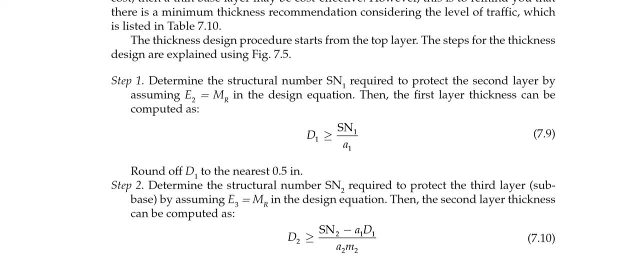 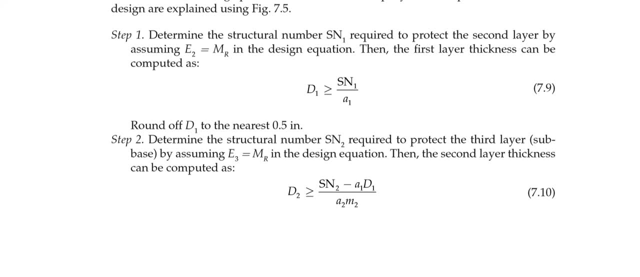 Yes, asphalt concrete, typically 6 inch, 6.5, this way. Then step number two: use E3 as your MR, Then calculate SN2.. Then use this equation, calculate D2.. Because you are calculating this, you know this part now. you know this. material properties. 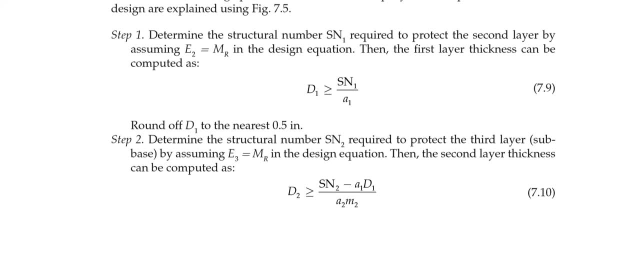 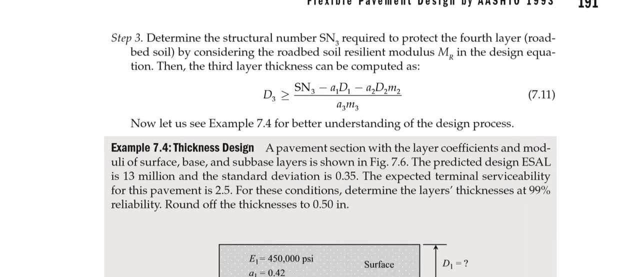 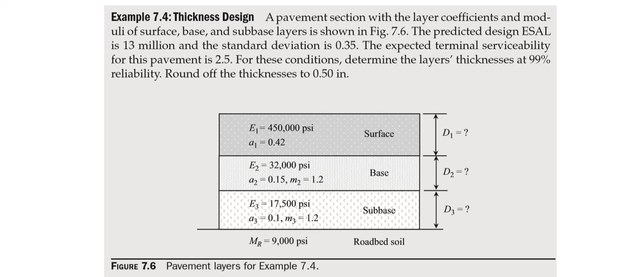 then calculate D2.. So this way you can calculate one by one. So hopefully you understood. If you did not understand, there is an example here. So this is the example given. Yes, my, this book. actually you know that I wrote this book. This book has so many example, everything is clear. 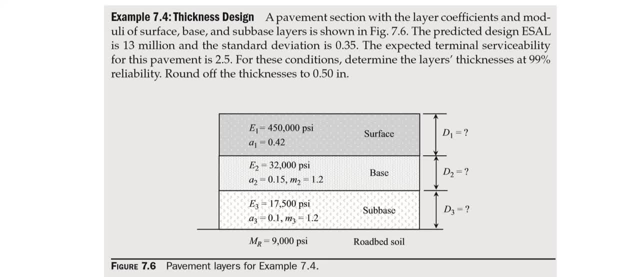 So this is an example here. Here you know the modulus of surface layer and A1, layer coefficient. what is D1,, D2, D3.. So many other values are given, whatever you need. So what to do? 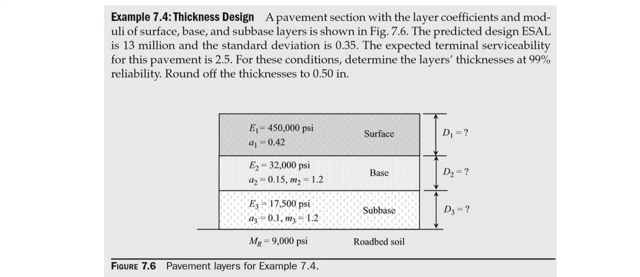 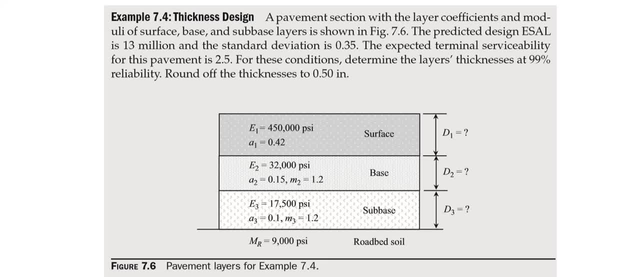 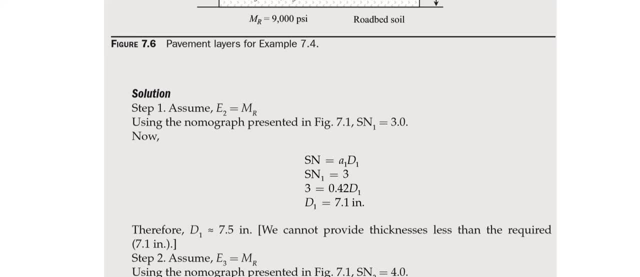 then use the nomograph and find s n. i found s n on 3, then s n on equal a 1, d 1 and s n on you, calculated from your chart 3, then solve it. you'll get d 1, 7.1. 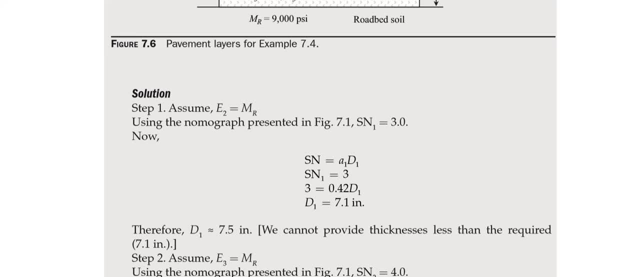 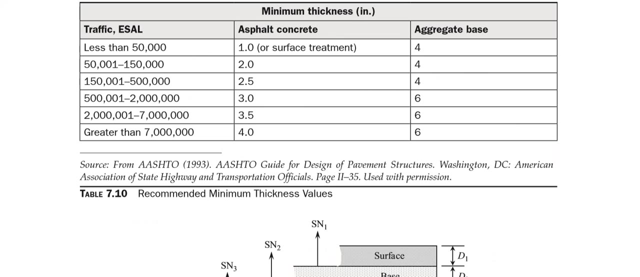 but round off to 7.5. now this should be more than the minimum value. so always check with the table which table i am going- again this table. so always check that your number is greater than this. yes, here maximum is like 4. i got 7, so way higher than that. 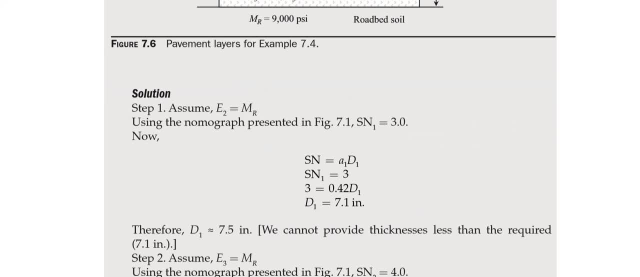 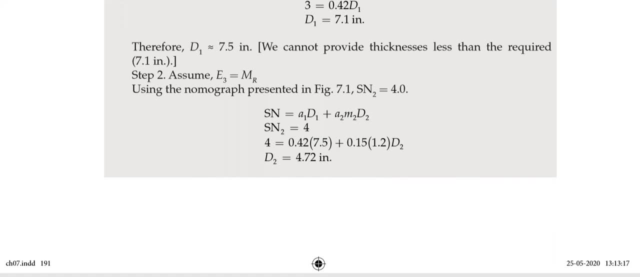 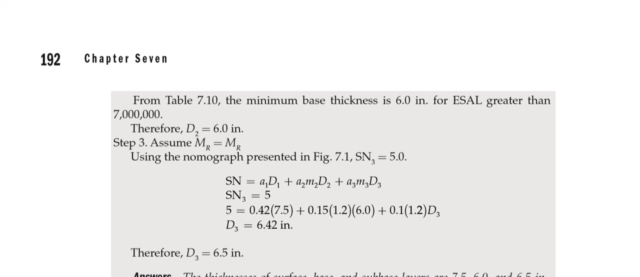 you okay, so this way you can continue. yes, a step number two, step number three. so in step number two i assume e 3 as mr and then calculated d 2, 4.72, round off to nearest hand number, and then step number three. so this way you can finish it. so i think hopefully you learned it.